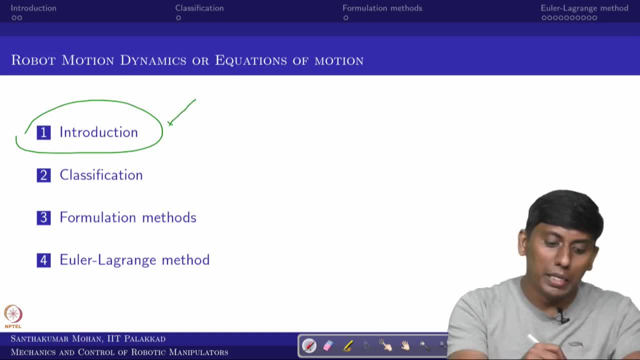 dynamics, The robot dynamics. again, in the beginning we said: So we can actually like write as a motion, dynamics and structural. So it is actually like structural. So both we are going to see, but this particular lecture is going to talk about more on motion, The 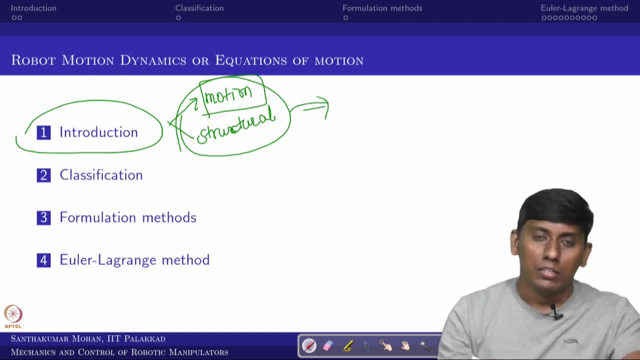 structural things will come in manipulated design aspect. So, however, this particular course is mechanics and control. So we would be seeing more on motion. So that is what we are going to give in this introduction. Then this motion dynamics can be classified. 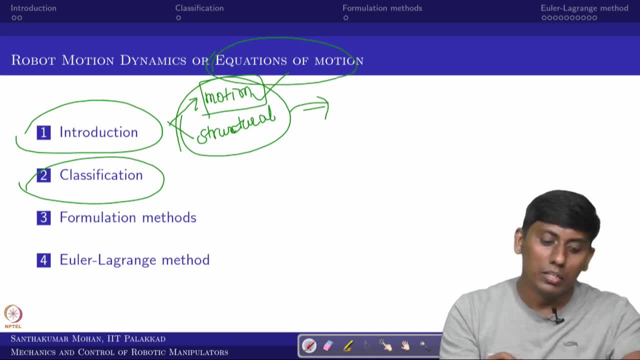 or this can be even some people called equation of motion. So this further classified into 2.. So that is what we are going to see. So how the forward kinematic model, inverse kinematic model, was there. then we have seen forward differential kinematic model and inverse differential. 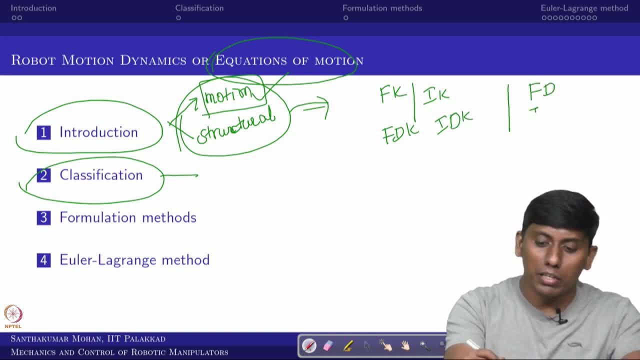 kinematics model. The same way we would be talking about forward dynamics and inverse dynamics, but the scenario is not the same. So here it is actually like mapping between you can say configuration space and you can say the joint. you can say operational space. 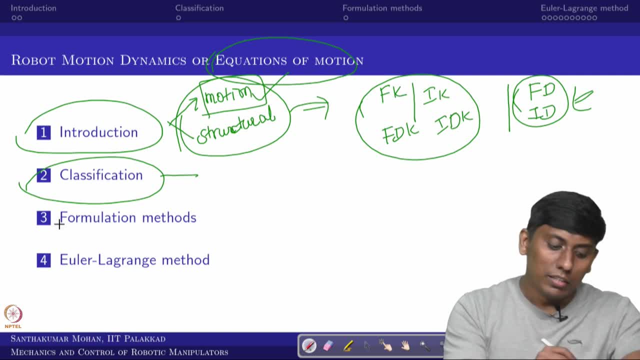 but here the spaces are different. okay, that we would be seeing. Then, for getting this equation of motion, there are several- you can say- formulation methods. we are going to talk about 2 popular methods in that. one we are going to see in this particular lecture in detail with an example. okay, So I hope now you are clear about the structure. 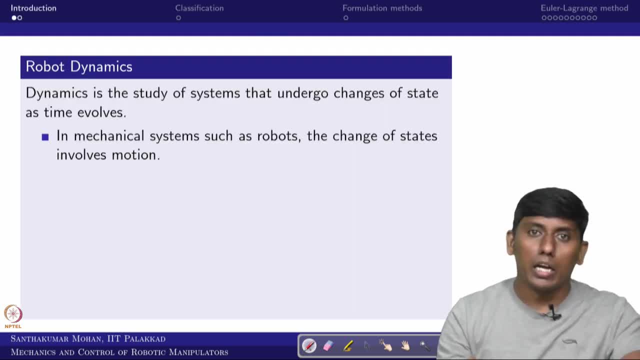 of this lecture. So we will go further. So you know, dynamics is nothing but The study of systems that undergo changes of state as time evolves. So in that sense the robot dynamics is more general. it would be having you call kinematics and the kinetics. 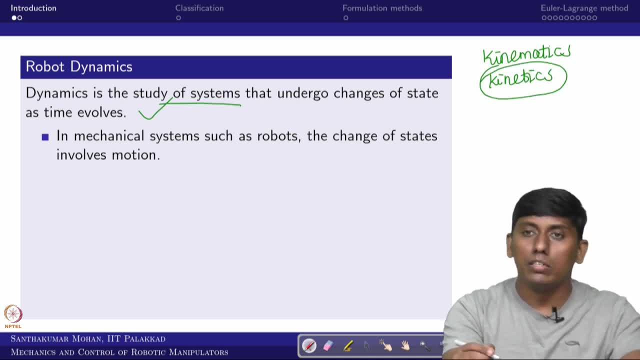 okay. So where one with regard forces are efforts, the other one is without, you can say constrain that. but here we are going to call as a general, in the sense you are going to relate the motion okay, And cause of motion or causes. So this relation we are going to relate, not like simple kinematics. 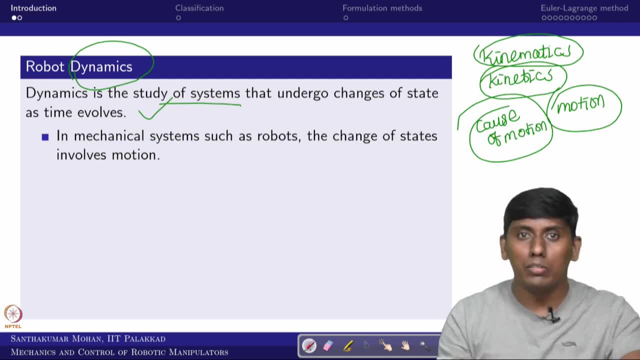 So that is why we always actually like robot dynamics kinematics. we will call robot kinematics, but robot kinetics is very rarely. people put it forward. So now, in that sense, what mechanical system also, such as robot, that changes of states involve motion? but what else would? 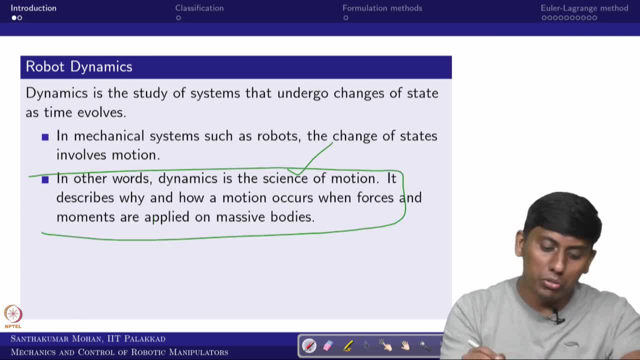 be coming. so it actually like you, science of motion, but it describe why and how the motion occur. that is what I said. so we are actually like relating the input to the output. okay, so here the input is actually like your efforts or causes- okay, the causes, which is 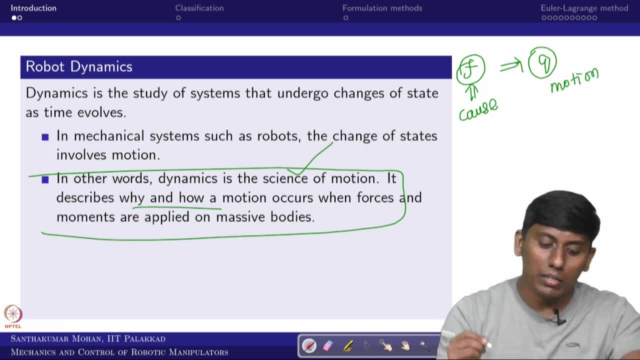 causing the motion and we are actually trying to see the motion relation. So but what it is actually like? a multi body system. so we are trying to see how it can be done one by one. so in the sense when forces and moments are applied on a massive bodies, 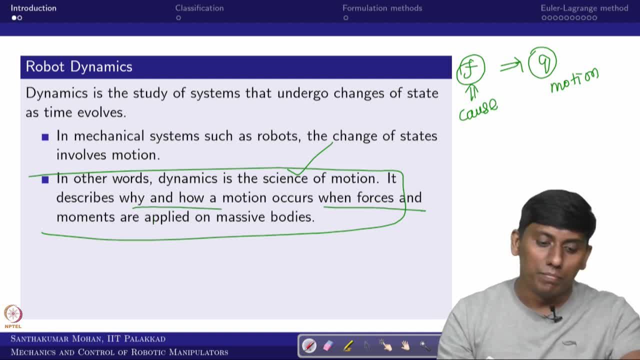 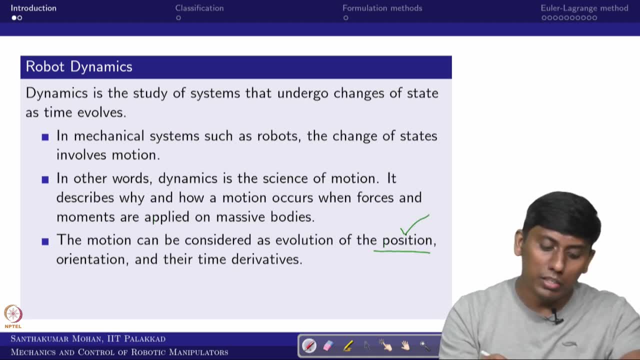 so how we can actually like understand the system of motion. that is what the idea, So why this is actually like very, very important because this is evolving from, you can say, position, so orientation. that derivative is actually like making- that is what I said- F equal to m? a. it is actually like Newton's second law, but if you take a very general 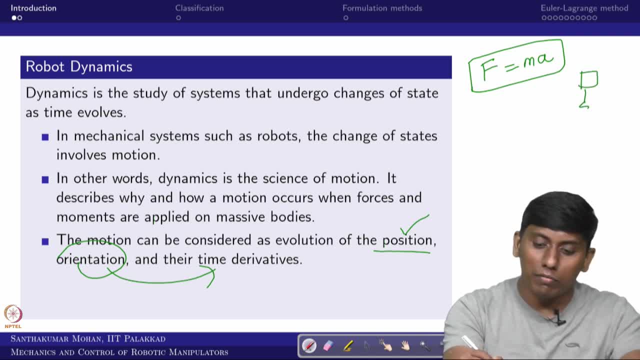 if you assume that there is a mass, that mass is actually like connected with the motion, with a spring that is connected with another spring and dash watt. So then you can see this would give a frictional component, this will give a restoring and this will give initial component right. in the sense, this same equation F can be written as function. 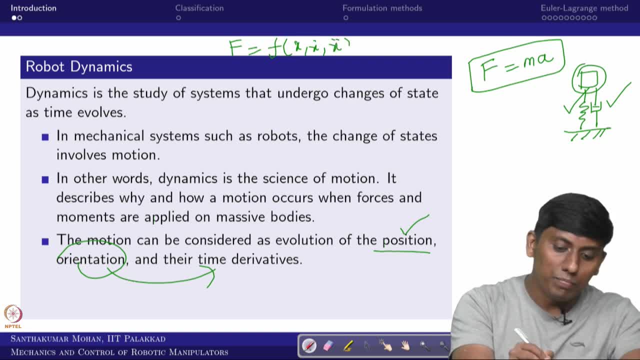 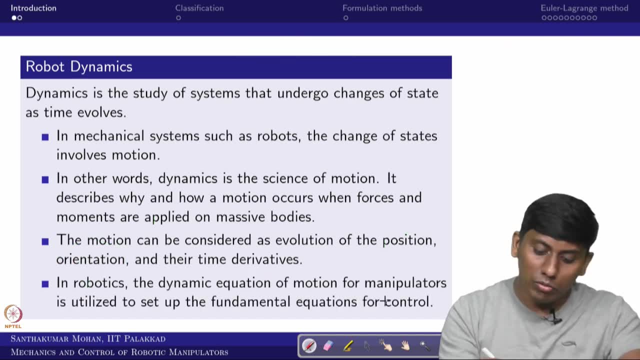 of x, x, dot, x, double dot. right? so this is what we are trying to write. that is what we have written here, okay? So, in addition to that, what? so this is actually like mainly to utilize, so two things. so it will actually like you. 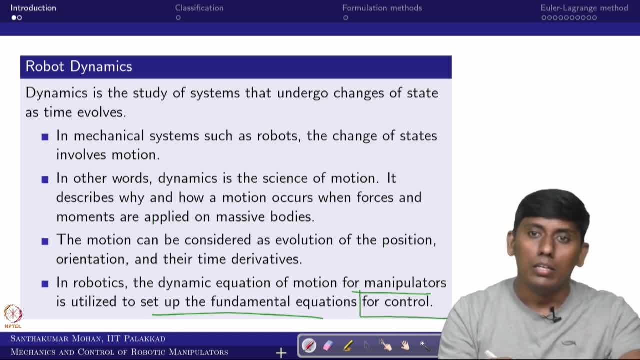 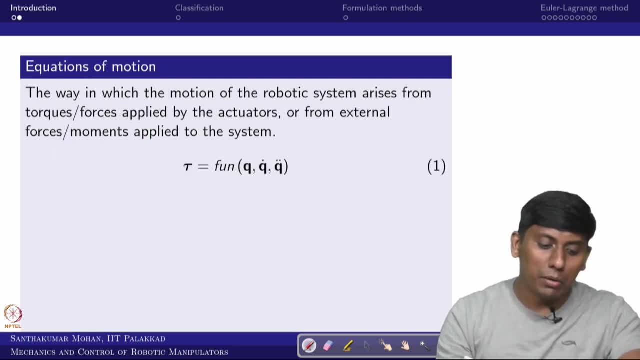 So this is a fundamental equation. but this equation is for control and it can be used for even what you call design, the overall system. So if you look at that aspect, so what one we expect? we are writing a generalized. so earlier I said F can be written as so function of you can say x, x dot and x, double dot. 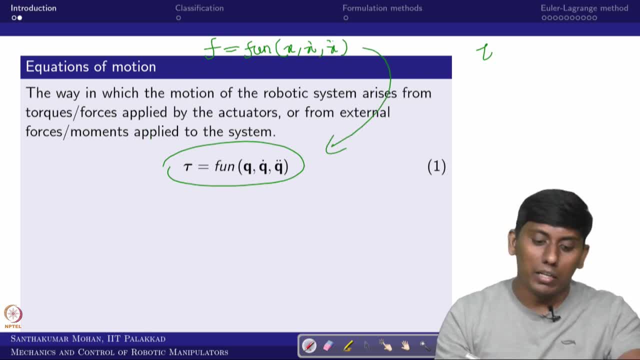 So this equation, we are actually like writing in a generalized manner with a vector. so this is actually: tau is the input vector And this q is actually, like you can say, the joint vector of joint variable, then the velocity and acceleration. the sense we are writing a generalized form, okay. 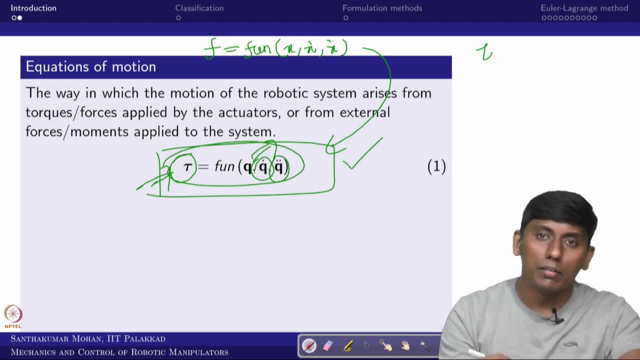 So this is more important for one, because this is a non-linear. so that is why we are writing straight forward. In fact, we have to write strictly. so q, q dot and q double dot, comma t, because this is a dynamic system, it is function of time, but we are actually ignoring, because q also 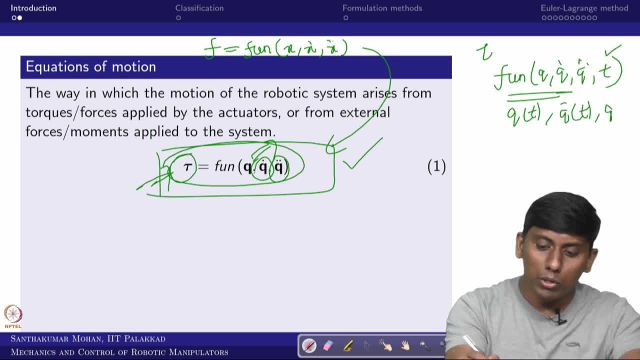 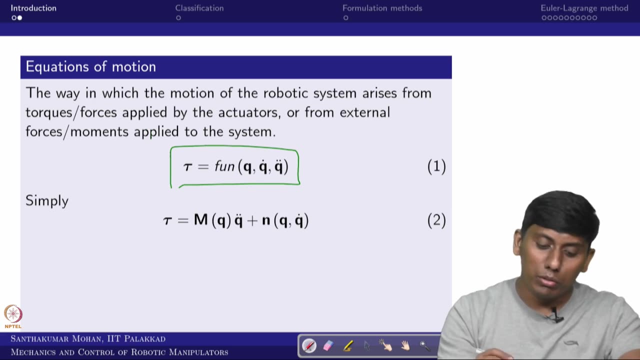 function of time. So q dot also function of t and q double dot also function of time. So we are actually like ignoring similarly, tau also function of time. okay, So that is the whole idea. So we will actually like see some people this bigger equation can be reduced into a small 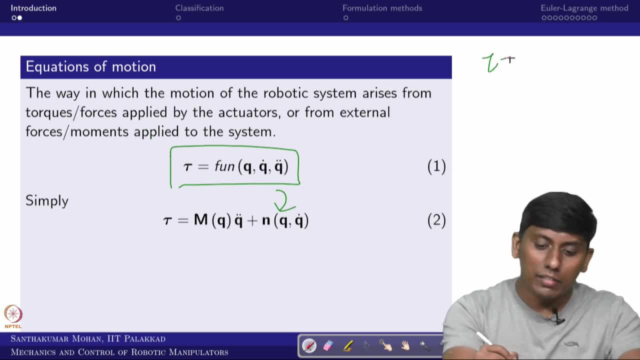 you can say state space form. that too, like we can write, as you can say acceleration plus other terms. So in the sense, acceleration coefficient will come as a matrix, So this is the other term- as a vector, and this is actually like acceleration vector. that is what we have written here. 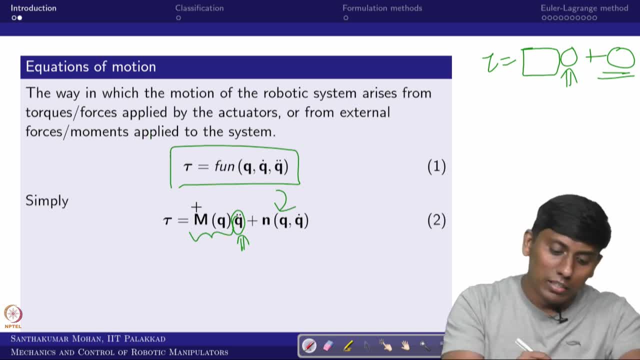 This is acceleration vector and the coefficient of acceleration vector is what we are calling as initial. So this is inertial matrix. okay, These all called other efforts, Even some people even further. this decompose into gravity and other effort. some people call even gravity frictional other effect. some people even further go on. 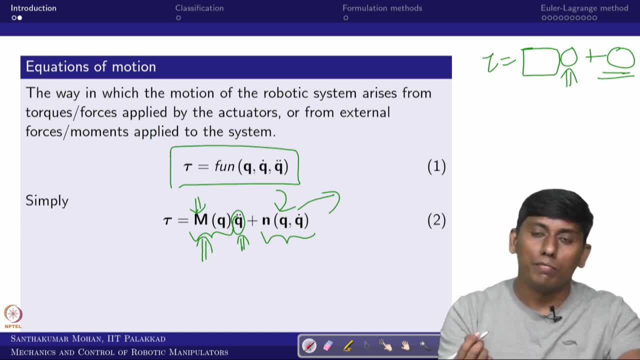 So centripetal and curl is separate And you can say friction separate, gravity separate, like that you can actually like make it. but I think we will restrict this up to this because we are going to do the second part as the simulation side. so I hope this would be very much beneficial, okay. 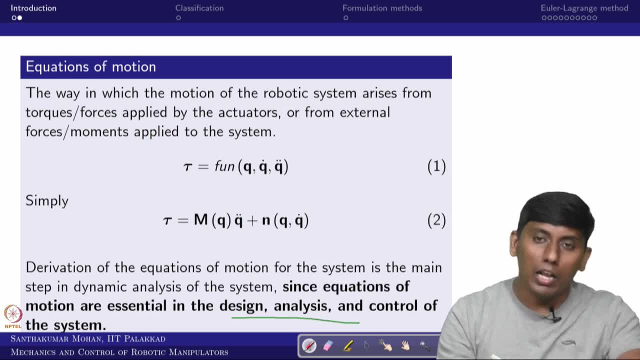 So why this is actually like very important? because it is actually like helpful for analysis and control and similarly, this can be used as a design tool- okay, in order to cross verify your system- and further use for design aspect. So that is why this is actually like very, very important. 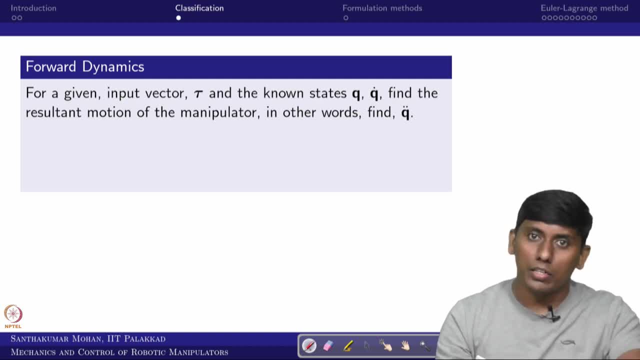 So now we will actually like see what are the subclasses of robot dynamics. So we have seen tau is actually like function of: so q q dot and q double dot, right? So these are the thing. so now this is actually like one space which is actually like motion. 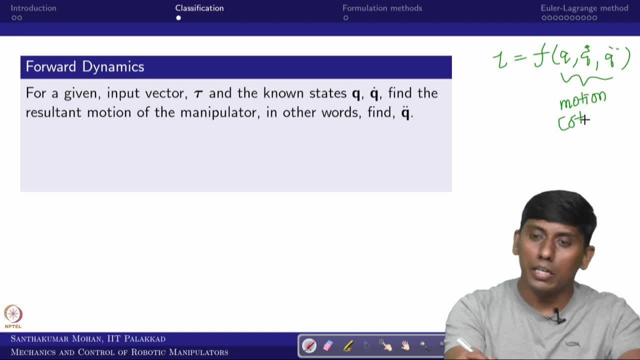 variable okay, which we simply call system state. So we call state variables, okay. So the other side is actually like what you can see, the input variable, in the sense it is the cause of motion, or you can say, simply called the causes, right, So can we map this causes to motion? so in the sense you take, you can say a serial manipulator. 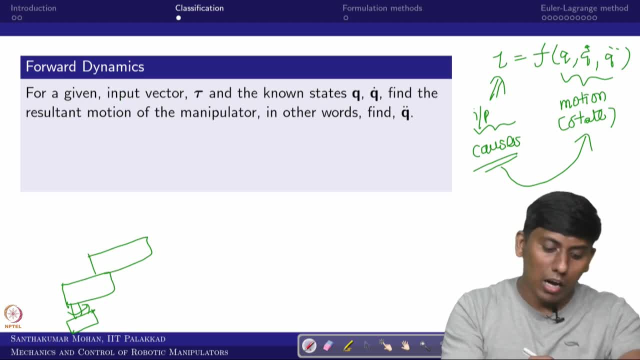 okay, you connect a motor and you provide a torque, how the system is actually like behaving. So if you look at that, so what you can see in the sense You are given a input vector, you are trying to find the you can say q dot, q, q, double dot. 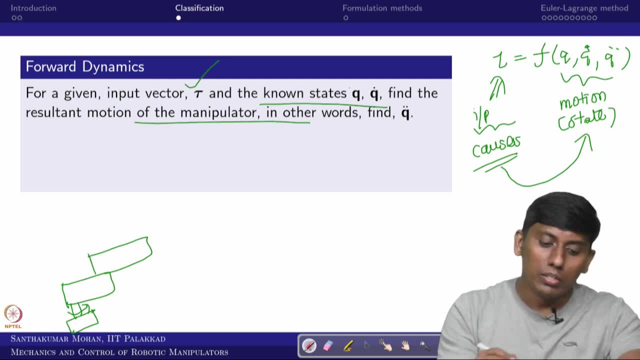 and q. we are actually trying to find the resultant motion. So, in the sense, so these are actually like known states: q dot q, double dot q. all are actually like we are trying to find out. in the sense, the input is known and we are trying to find out. this is what you call forward dynamics. this is very simple. 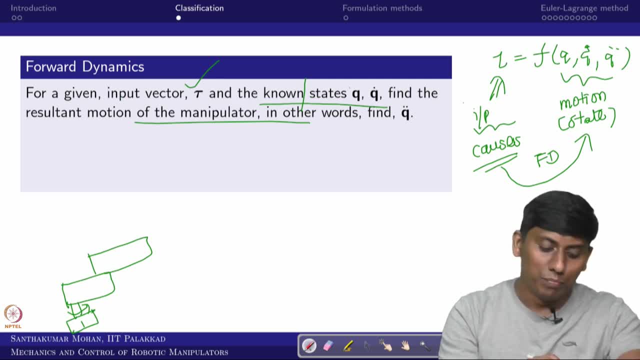 So you have a motor and give a torque. So you have a motor and give a torque, So you see the system. or you have a linear motor, So you are actually giving a force and trying to see how the system is behave. the sense it is actually like forward dynamics. 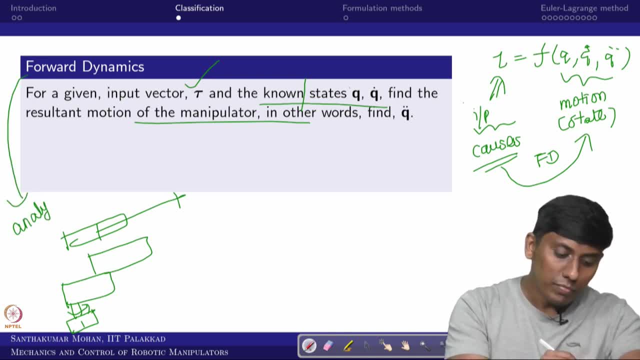 So what it is trying to do, it is actually like analyzing in real time, it is actually like analyzing in numerical background, it is actually like simulating, right? So that is what the whole idea, which is very similar to differential kinematics, but differential kinematics is mapping between what 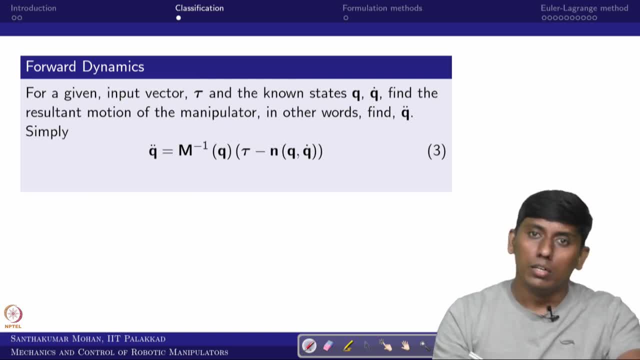 Okay, So task space velocity to configuration space velocity. but here it is mapping the input vector to what you call the unknown q double dot. then you can integrate, then q dot will come. Okay, So that is why I said that known state q and q dot. you are trying to find out q double. 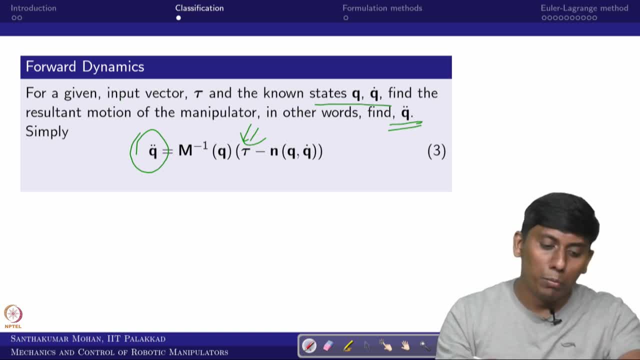 dot. this is forward dynamics. it is very close to open loop. you can say analysis system, not control. you are actually like giving input and see what is the system output, In the sense there is a football in front of you, Okay, You just go and kick. 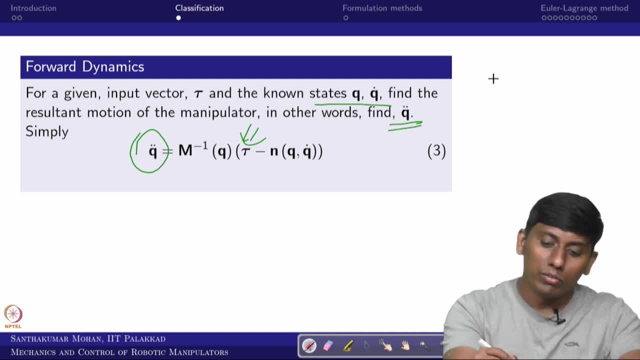 So how the ball is rolling, that is what you are trying to see. So this is actually like something like you have one ball and you are actually kicking it, So the ball is rolled, that kind of thing. Okay, So this is what you can see. simulating or analyzing the manipulator. 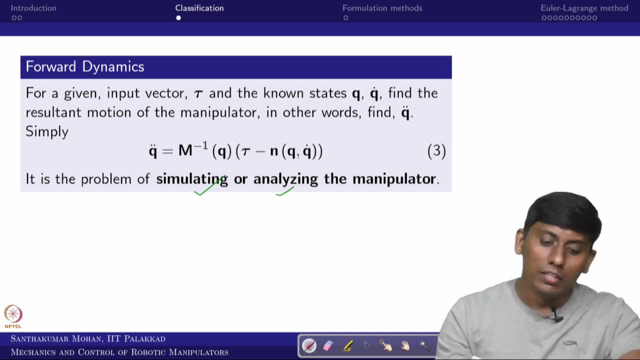 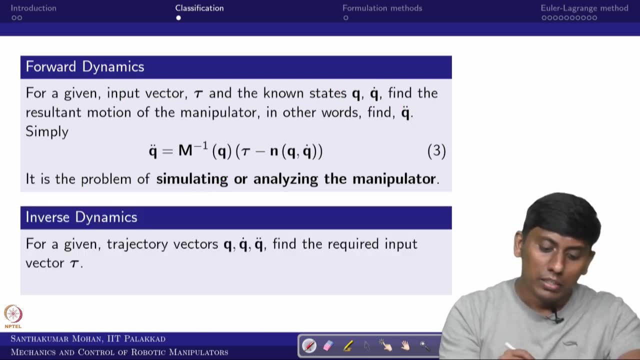 So obviously the contemporary of this is just opposite side, where the q, q dot and q double dot are would be known, and you are trying to find out what is done. Okay, So in the sense, these are actually like given as a trajectory, Okay. 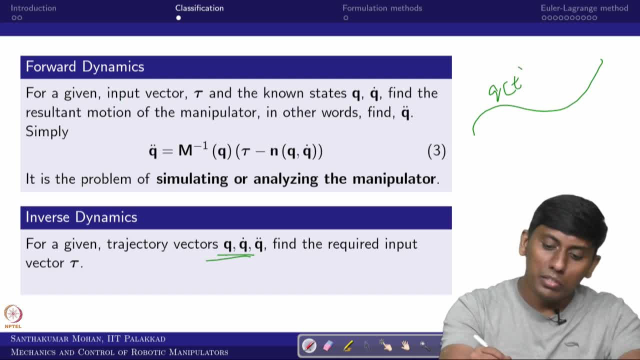 So in the sense it is actually like time based trajectory, So which is actually like twice differentiable in the sense q dot, q, double dot would be known in the sense you take a car and you are trying to follow this with respect to time or in 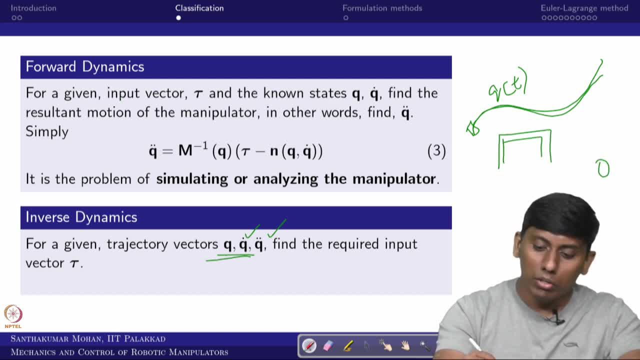 the other sense. So you have a ball, that ball need to go at a certain goal post, Okay, So this kind of thing in the sense. so how much force are, what direction you provide a force, the ball will roll here, Right. But the other thing is it is open. 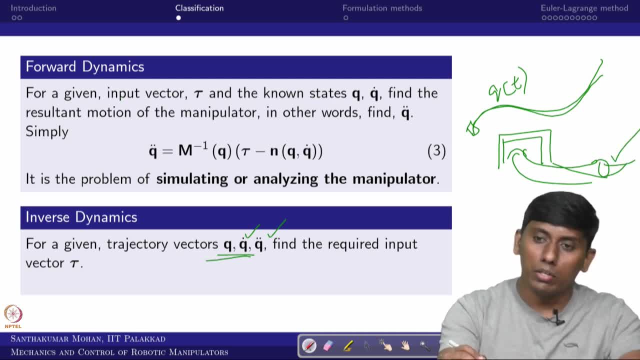 You are just hitting and seeing the sense you give a known input, known force, and seeing the rolling of the ball, which is forward dynamics, whereas the inverse dynamics the ball supposed to go in certain manner. So what force and direction you need to provide? So that is what it is, more or less a small kind of controller, but it is still open loop. 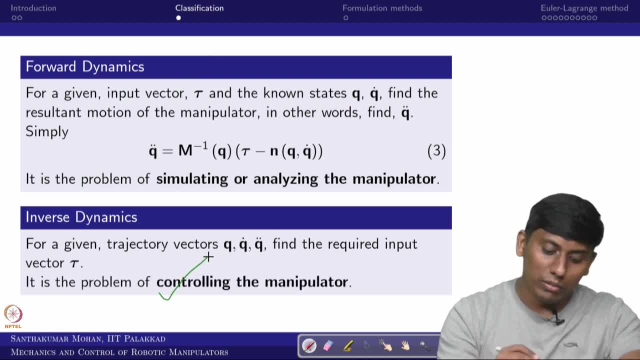 controller. It is a feed forward, Okay, So that is what we are actually like trying to see. So this is a problem of controlling manipulator, But this is a problem of simulating Or analyzing the manipulator. Okay, I hope you would be clear now. what is the classification of? you can say dynamics. 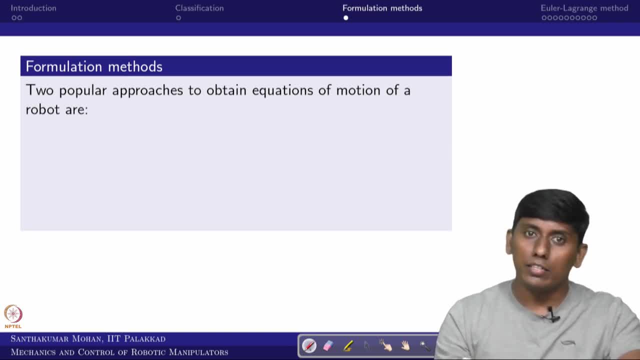 Now we will see what are the formulation methods. So there are several methods, as I already mentioned, but we would be taking two popular methods or approaches which would be useful for the equations of motion or equations of motion of a robot or manipulator, which is very common in rigid body dynamics. 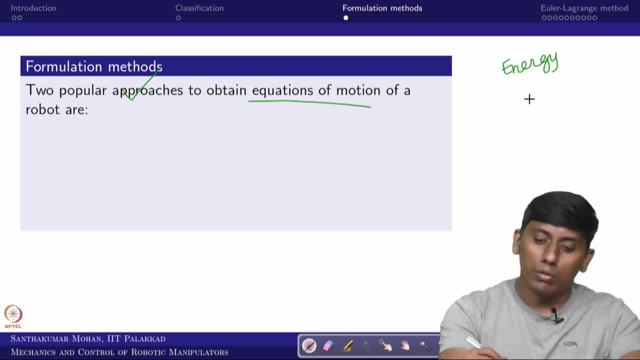 So one is actually like energy approach, Okay. So the other one is actually like equilibrium approach, Okay, So that is what we are actually seeing it, Okay. or some people call that is momentum approach. So one is energy based approach, is Lagrangian Euler, where Lagrangian is actually like modify. 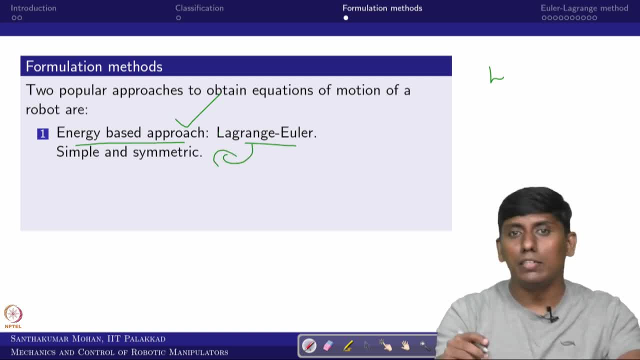 the Euler equation and come up. This is very, very simple and symmetric in nature And it actually give much, much better result for a small, you can say, size of manipulator with very less number of elements, Okay, Whereas the degrees of freedom is actually increasing, in the sense the active joints. 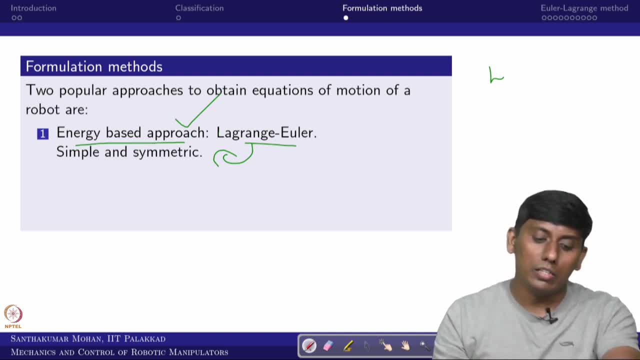 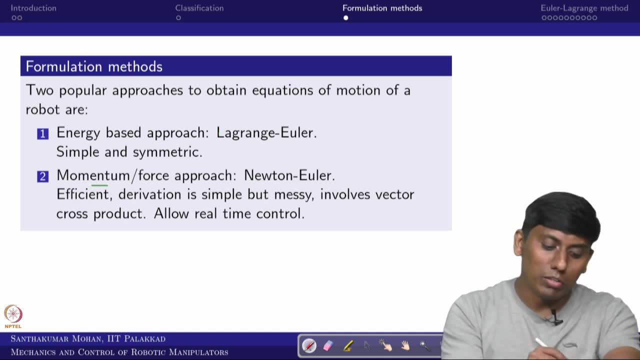 are actually like getting increased. So the Euler Lagrangian is not so easy or Lagrangian Euler is not so easy. Okay, And the second thing is. the second one is momentum force approach where Newton's- you can say second law and Euler's you can say equation of motion, can be used. 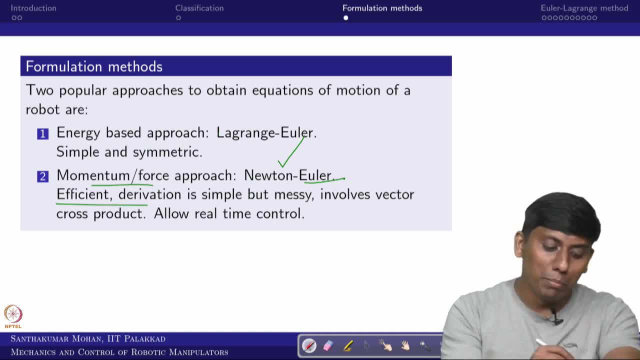 So this is very efficient in terms of computational aspect or implementation side, because the derivation is simple. But this would be consist of partial derivative and time derivative, but here there is no derivative involved. Okay, So that is why most of the people uses for real time control the- you can say Newton, Euler. 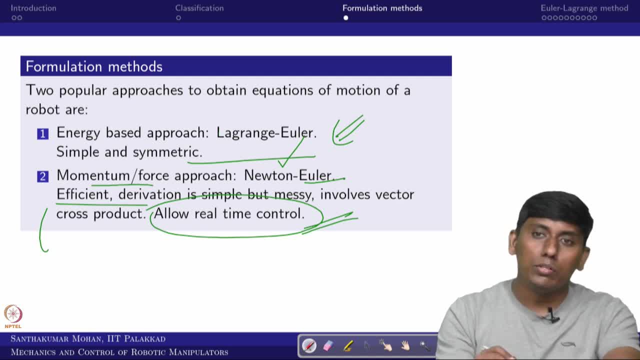 approach rather than the Lagrangian Euler approach. Only issue is this would be having a vector cross product. but it is actually like messy. you have seen already the velocity propagation, right, you have written. so omega 1 to omega n, then v1 to vn. 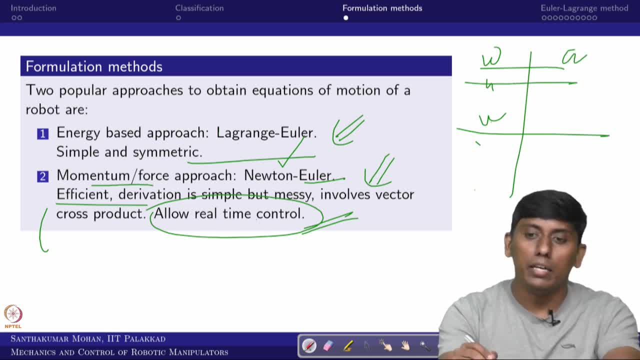 Okay. So similarly in this case it is supposed to go a0 to an, then you have to go for the body, then you have to go for acg to you can say ac0 to acn. Then you have to go for inertial force. inertial moment, it is actually like lengthy but computational. 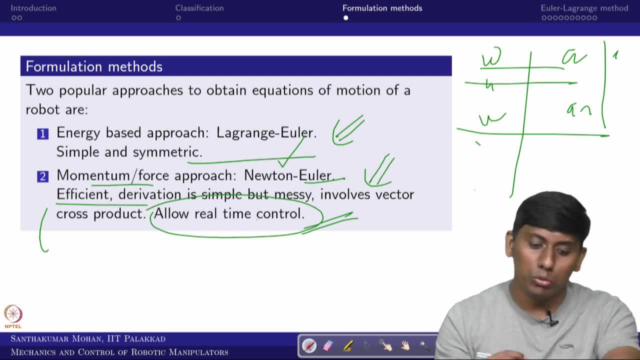 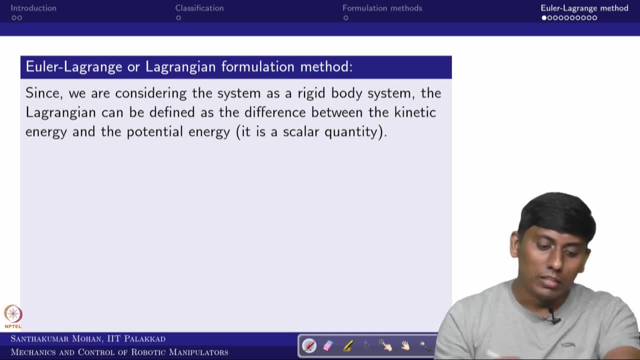 side. although it is a lengthy, it is actually, like very efficient and easy to implement. So let us actually like go to one such method in this particular lecture. the second method we will see in the next lecture. Okay, So Euler Lagrangian is actually like. as I already mentioned, it is energy based approach. 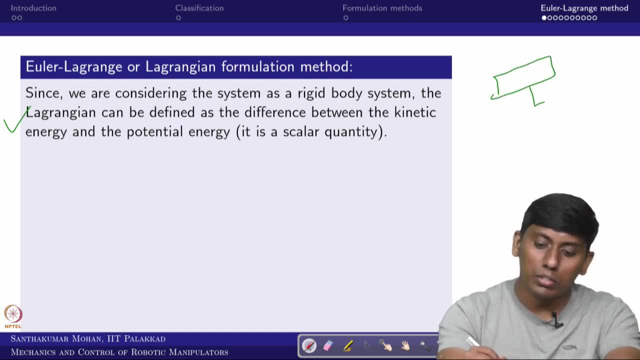 but in the beginning of the lecture itself I said this particular course we are talking about only rigid body. So in the sense we are talking about rigid body dynamics. So since the system is rigid, so what are the energies would be there. So only two kind of energies would be there. 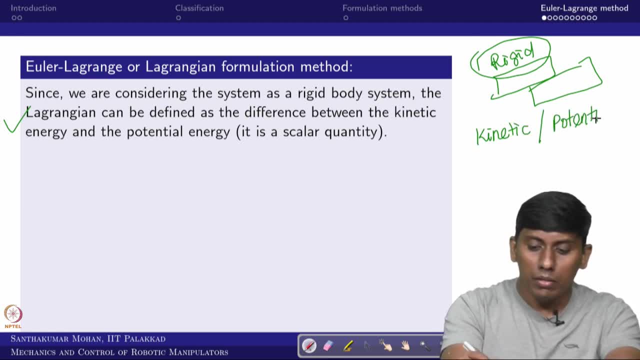 So one is kinetic, the other one is potential. Okay, So these two energy, if is there any difference between these two energy, Okay, Then there is a motion. exists even this energy difference how they have written. So kinetic energy is always upper hand. 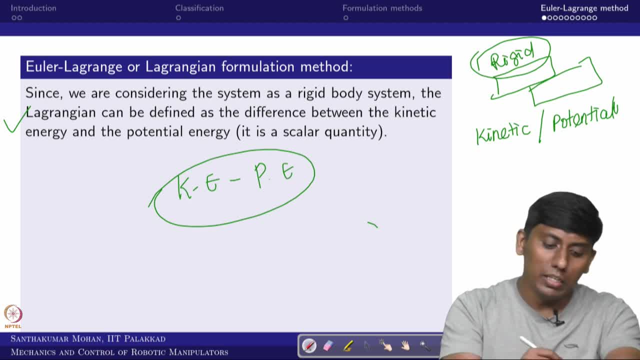 So kinetic energy minus potential energy. if there is a quantity, that quantity is a scalar. if there is a existence of this quantity, then there is a motion exists. So based on this L value, we can calculate the equation of motion. that is what the Euler, Lagrangian or Lagrangian formulation method some people call Lagrangian Euler method. also. 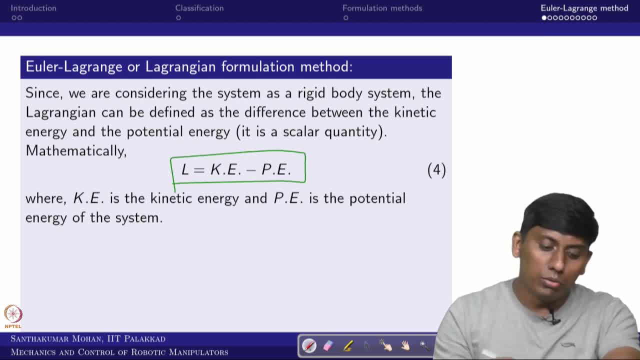 So that is what we are seeing it right. So now this energy difference, what we are trying to use So further, the equation is actually like coming based on very simplified manner. The detail is already given in some of the lecture handouts. you can see how this equation 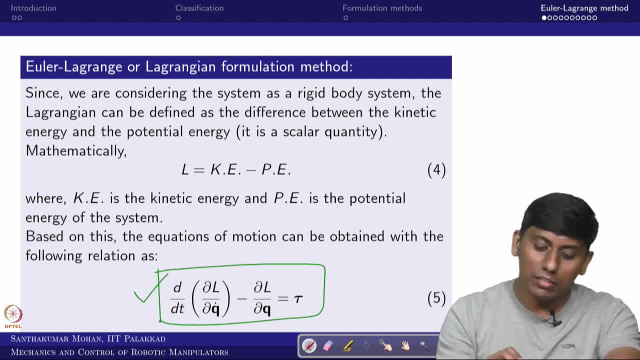 has come. Okay, So right now we straight away take this equation. This equation has come from the modified energy. you can say equation so you know if this is 0. So that would be the energy conservation. but right now we are giving the input, that is. 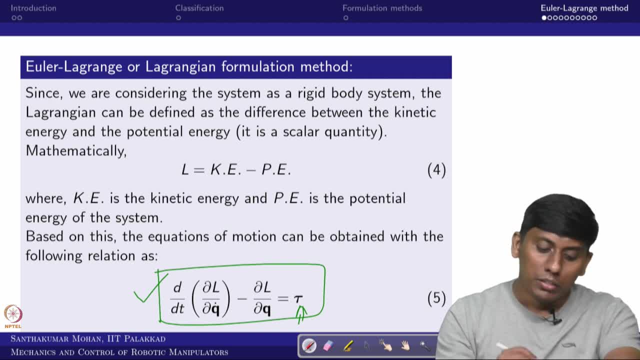 a modification, as done from the energy method. Okay, So now you can see that L is the scalar, but the q dot is actually coming in the other sense. So tau i, I can write as time derivative of so dou L by dou qi. okay, dot, this is a dot. 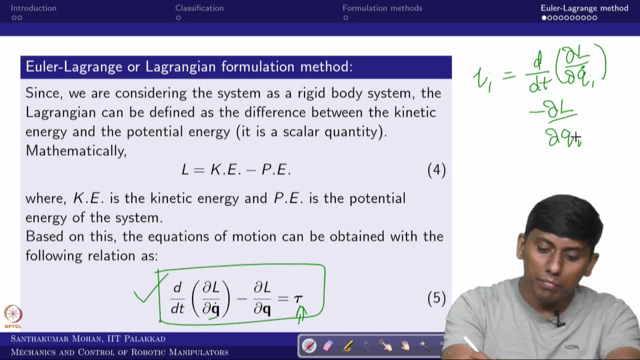 minus dou L by, so dou qi. okay, So that is equal to tau i. So this you can recall. this is a vector form I have written, but this is actually like individual element, you have to do it, okay. So just to give idea. so I am just giving a general expression. 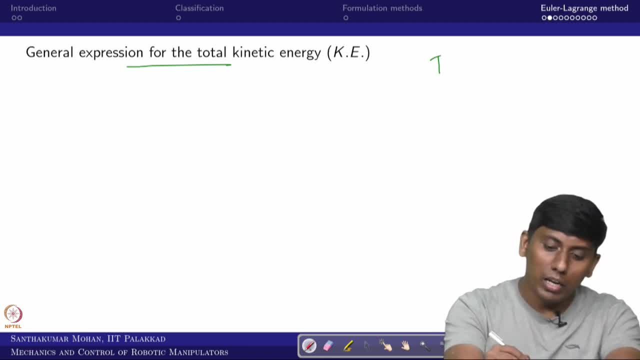 So where the kinetic energy would be having two parts. So one is actually like translational kinetic energy. this is due to the mass, okay, So. then the rotational kinetic energy: that is due to the second moment of inertia, okay, So or you can say simply inertia. 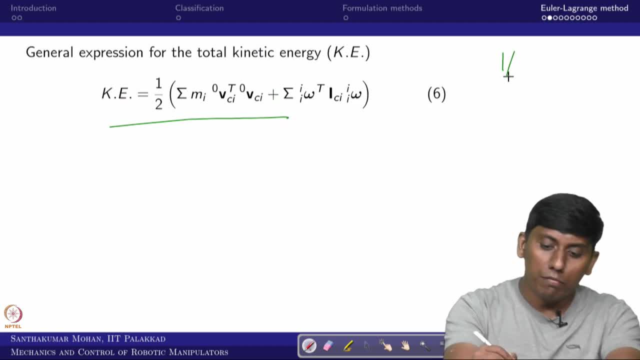 Okay, So that is what we are trying to write. So you know, half mv square is a scalar form, that you want to write it in a vector form, So v. transpose m into v, so half would be common. Similarly, if you write i omega square is the scalar form, so the same thing, you write it. 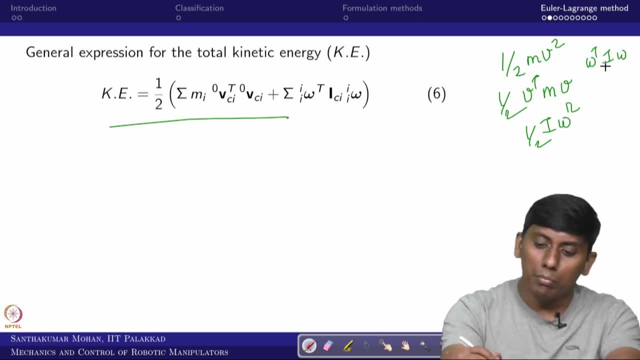 vector form. omega transpose: i is the matrix and omega so this one. So this is a tensor. okay, the tensor. we would be using it, so that I hope you are already gone through what is tensor. So this is a inertia tensor and this is the- you can say- translational inertia, which is: 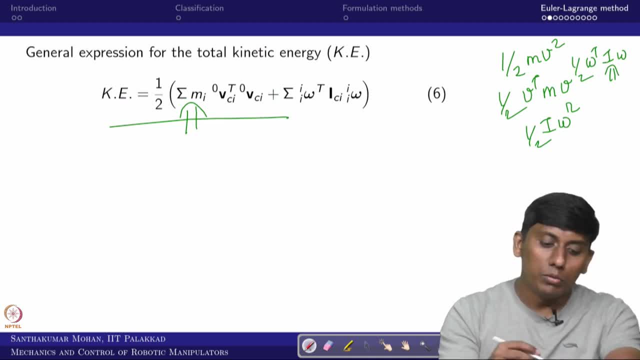 a mass. as a scalar you can take it out. So one thing you should be knowing. this is actually like ci with respect to what you call zeroth frame, in the sense the absolute velocity, and absolute you can say what you call acceleration. we would be using further on, okay, but here it is actually like only 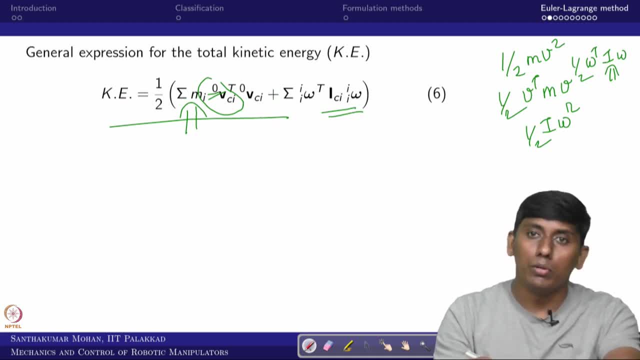 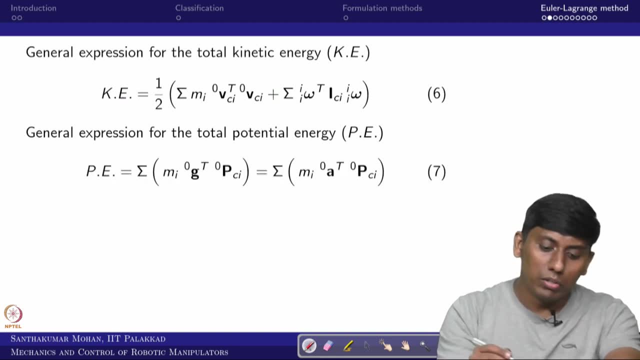 corresponding angular velocity. Okay, But this is actually like absolute. that is what one supposed to be known, okay. So let us actually like move further. so this is what the you can say potential energy, which is mgh, but this h is actually like you can write it in a position vector: the vertical. 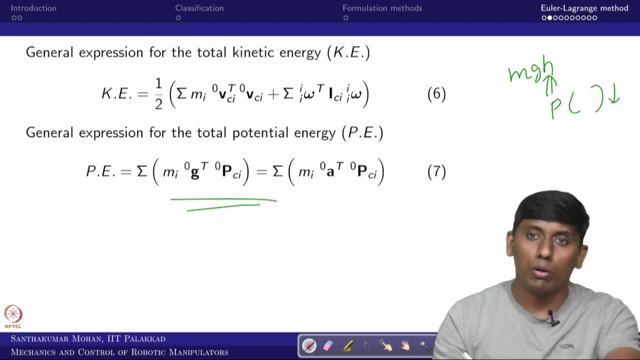 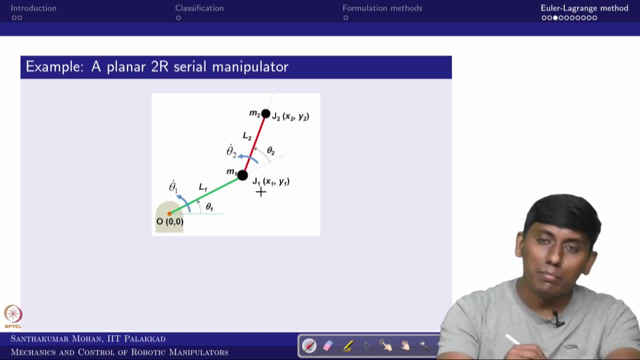 axis, which axis you are considering the gravity that axis you have to take it. okay, So now, in that sense, we will take it. one simple example. I assume that this is a mass, concentrated in the sense. So here, what will be equal to X, 1 is plus a short term. 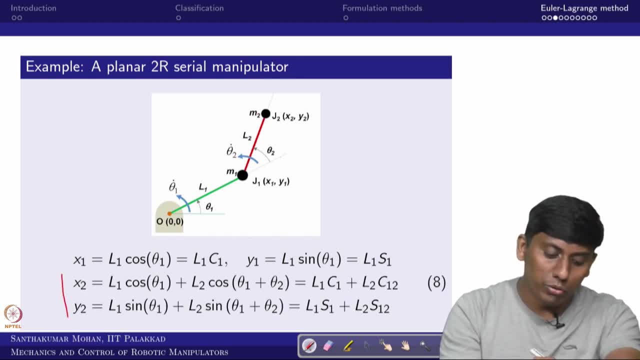 It is like r over c. So tomorrow what? this is going to be Okay, So now you do not actually like can do. you can do x1 dot, so y1 dot, similarly x2 dot and y2 dot and half m, x1 m1, x1 dot. 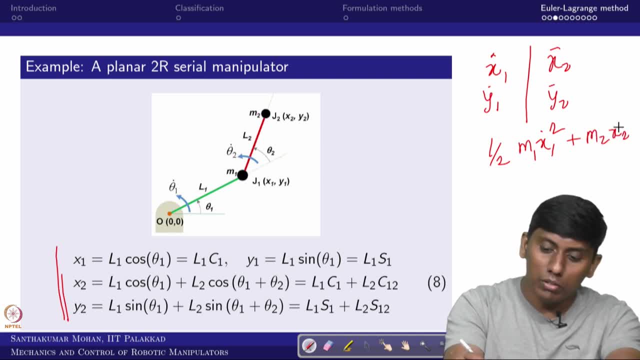 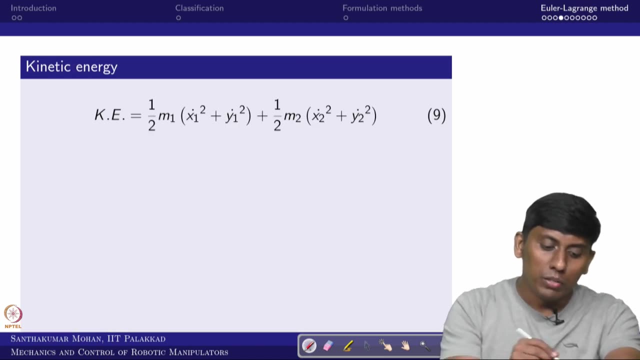 square plus m2, x2 dot. square plus m1- y1 dot. square plus m2- y2 dot, square right. So this you can actually like, calculate, and then you can find it. that is what we are trying to do. you can see so far that you need to know x1 dot, y1 dot, x2 dot, y2 dot. so you know. 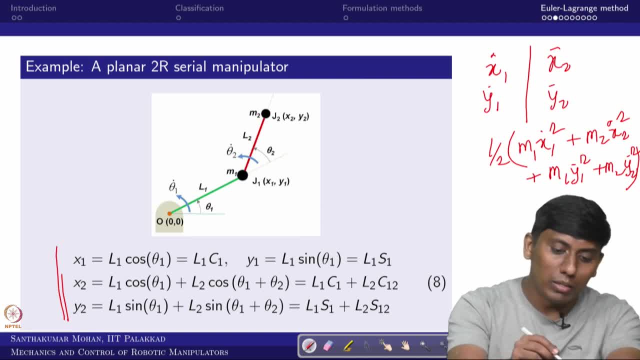 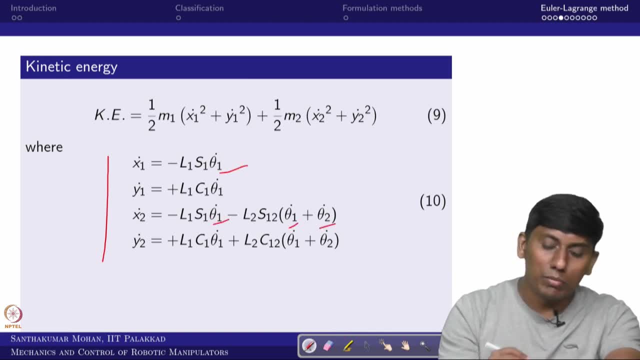 already x1 and x2, y1 and y2, so you can actually like take time derivative. so this is what the time derivative, so that would be function of. you can see the joint space variable. So now you can actually like substitute that you will get the kinetic energy in this form. 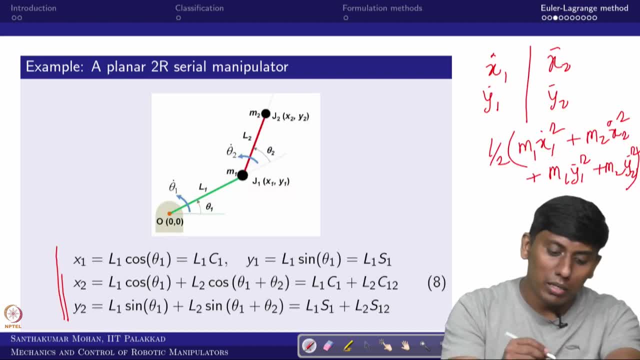 and you can take the potential energy. so here you can assume that the gravity is pulling down, So in the sense the gravity direction coming down. so you can actually like see in that sense, so y1 is equivalent to h of the first body, so y2 is actually equivalent to the second. 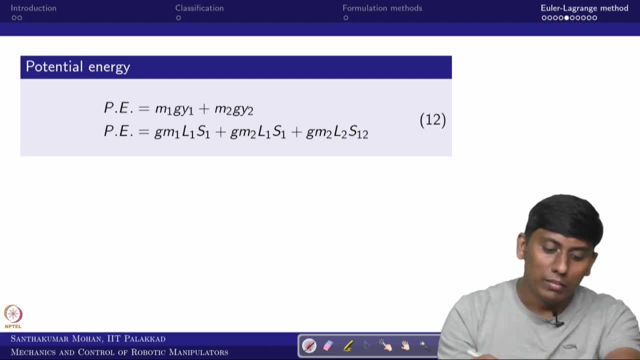 body right. So that is what we are actually like trying to write so you can see like m1 g y1, so m2 g y2, so that original value we substituted. So now what we got? potential energy, we got it previous slide. we got the kinetic energy. 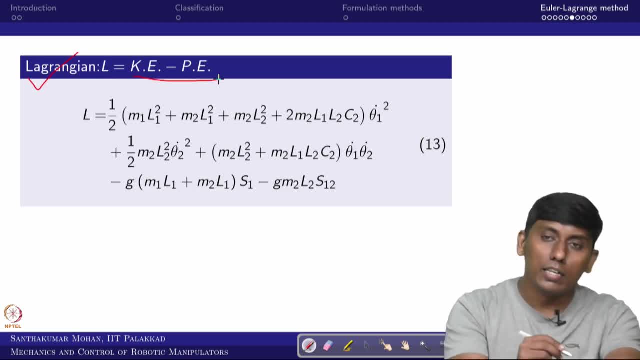 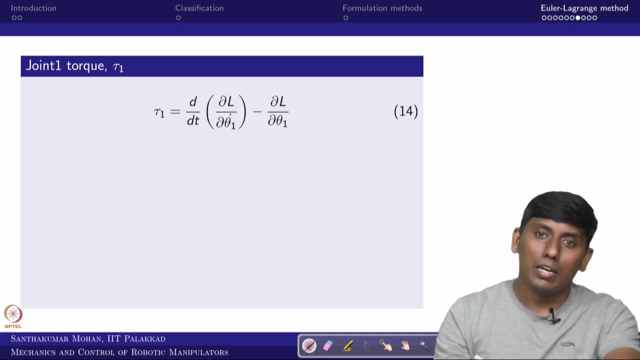 now we Take the Lagrangian, which is kinetic energy minus potential energy. this give this a scalar, So now we can actually like substitute the relation. so what relation? if you want to have a tau 1? so tau 1 is time derivative of a partial derivative dou L by dou theta, dot 1 minus. 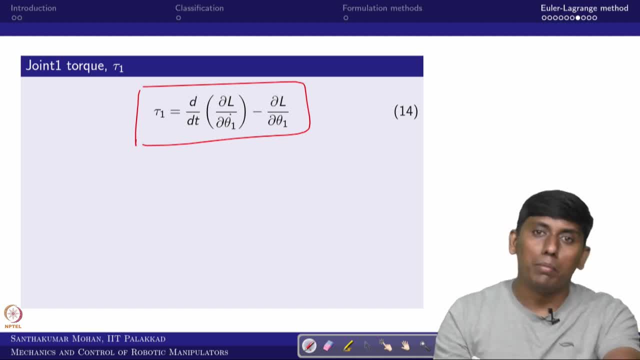 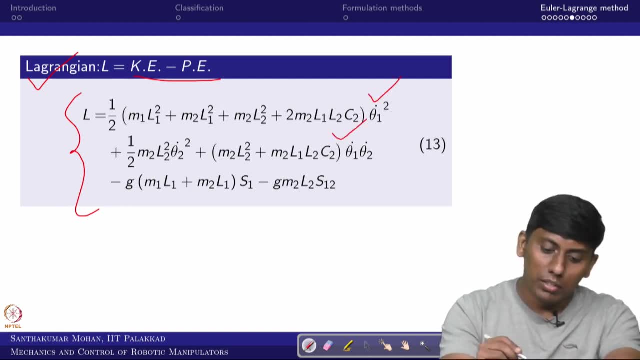 dou L by dou theta 1.. So first we calculate dou L by dou theta 1. so far that you can just recall, this is what. so theta 1 dot is in this term, So this term and these terms are 0 right. So in the sense this 2 goes, So this goes out. and here you. 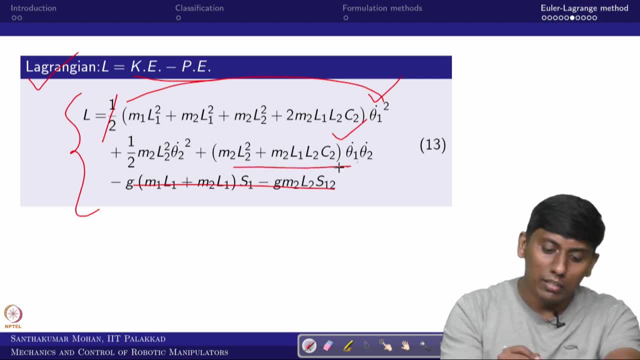 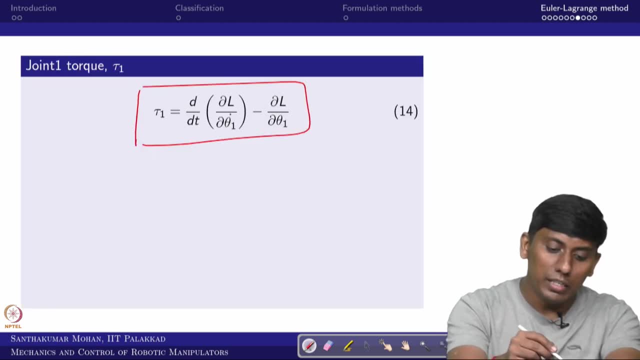 can see like this: theta 1 dot is coming only here, So this goes out. So in the sense, theta 2 dot remain here, theta 1 dot remains. So we can see what is that partial derivative right right. So similarly you can take dou L by dou theta 1.. So unfortunately here. so 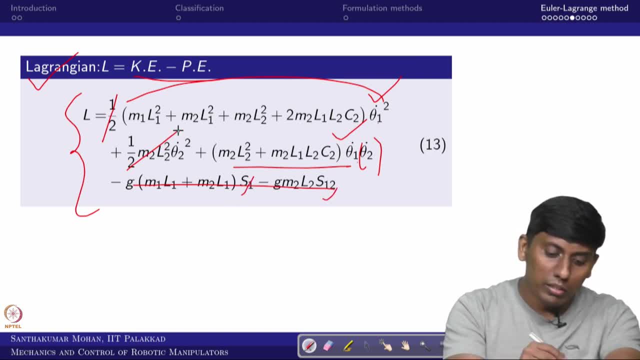 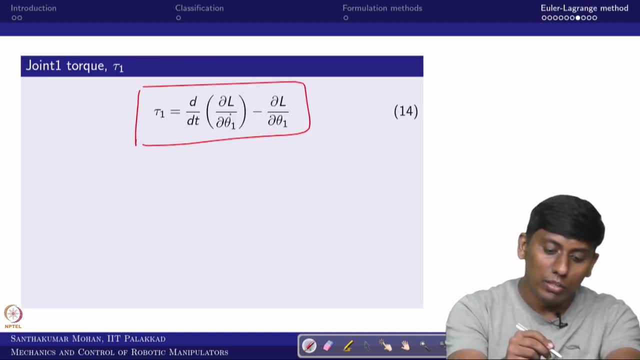 theta 1 is here, So theta 1 is here. So in this 2 equation nothing. So you can take it 0 and these 2 equations are. these 2 relations are coming, So that is what you can actually. 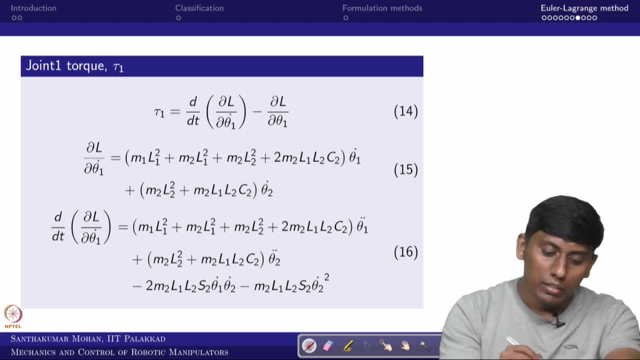 like, take it, ok, This is time derivative you have taken. So this is actually like partial derivative. you take a time derivative and then you can see: this is what you can see as dou L by dou theta 1 right. So now this is known and this is known. So you just directly. 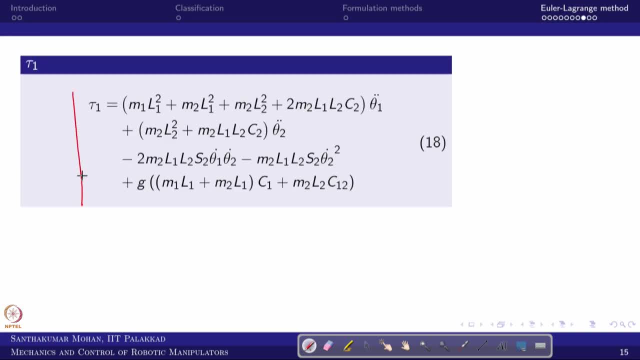 subtract this, So that is what your tau 1 right? So tau 1 once you obtain, So whenever we do, you can actually like cross verify. So what cross verification? you have to see any equation, for example, A equal to B plus C, plus you can say E into F. So what supposed to be? 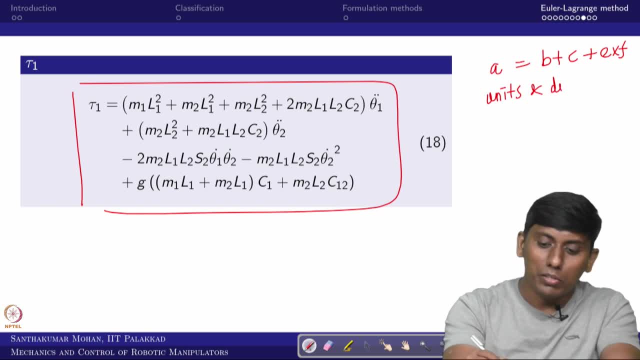 the units and you can say dimension should be equal. So in this case it is a scalar which is all 1 cross 1.. So this tau is actually like Newton meter, right? So then? so inside any term you take, 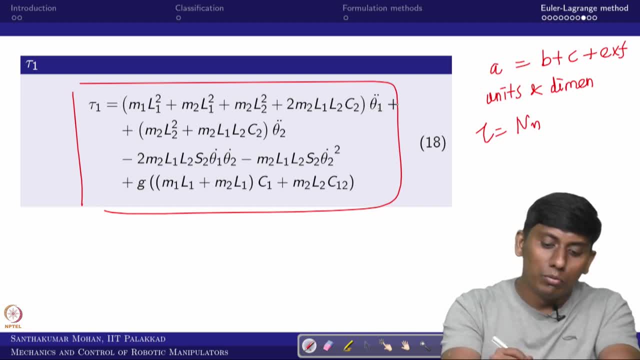 it should be Newton meter right. So what this will give. this will give radian per second square. So in the sense you can actually see what is Newton meter. you can write So kilogram right, meter per second square, into meter. the sense: kilogram meter square per. 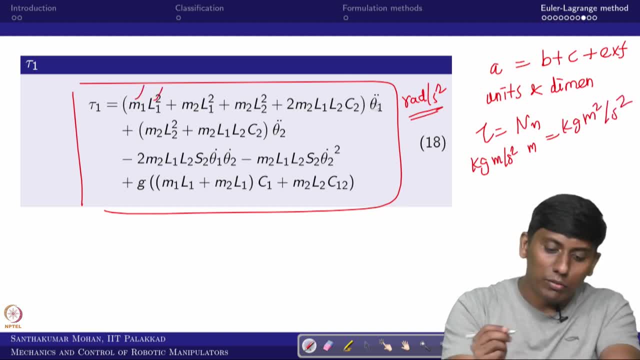 second square. So here this is kilogram meter square and second square is there. So this is kilogram meter square and second square, like that you can see right. So in that sense, if theta 1, double do Dont come, so then you have to see the other side. So some kilo. 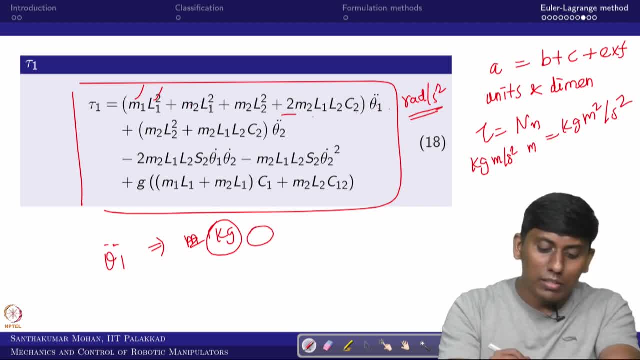 gram should be there. some mass and 2 distances or one distance square should be there. right that you can cross check if theta 1, dot square comes, or so theta 1, dot, theta 2, dot comes, so then you can see that this is already equal. 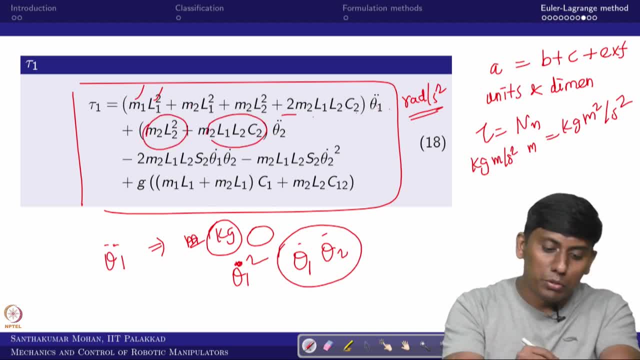 to again radian per second square, so you can see the same thing supposed to be there, right, you can see one. you can say mass, and two, you can say distance. you can get it right. so, similarly, here the gravity is there, which is meter per second square. right, then you can see like: 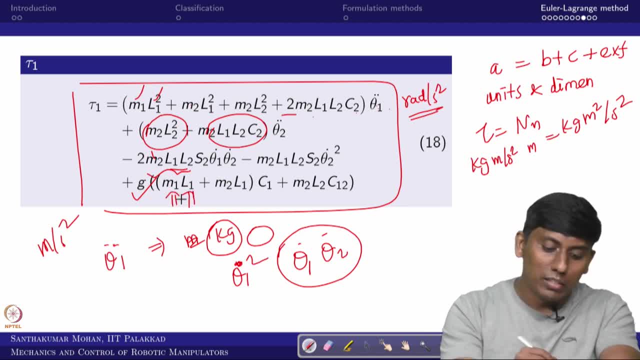 only one meter should be there, the sense, one length and one mass, so you can cross check. so like that you can always cross check and then you can actually like get it. so when we write this in a matrix and vector form, even one more check is there. but whenever